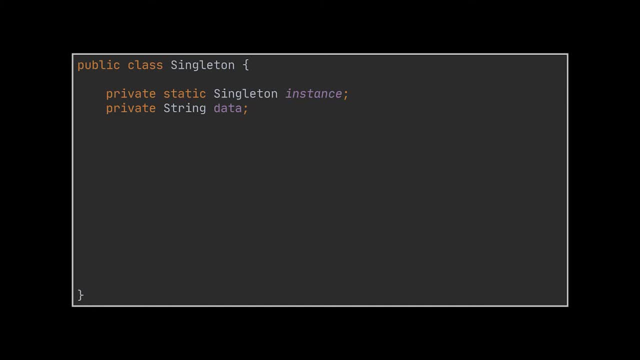 Under this instance, you can go ahead and add the attributes of your singleton class. In case of a database, these attributes can be the username and password needed to connect, for example, or anything else. Now what we need to do is add a constructor to create an object based on this class. 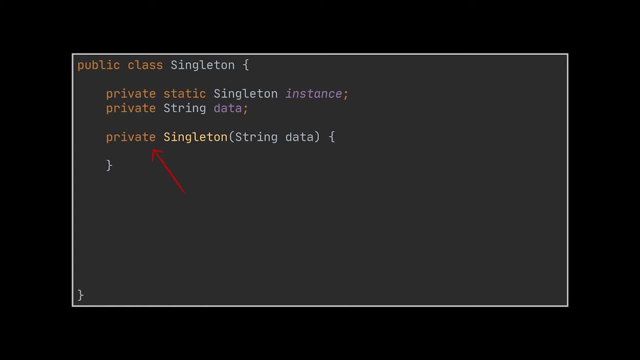 Make sure that the access level of this constructor is set to private. Inside this constructor, we can go ahead and create a new class. Inside that class, we can go ahead and initialize all the attributes of our object. here, In my case, we only have one: the data field. 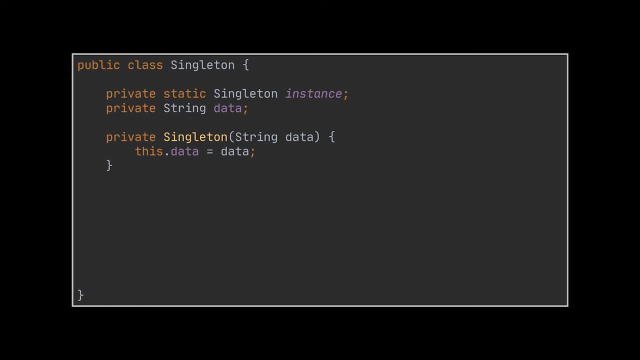 This constructor was FlowerTwit, because we only need access to it via a public static method created inside singleton. Usually that method is named GetInstance to refer to the same single instance it returns, So this method should return an instance of the Singleton class, the instance we declared. 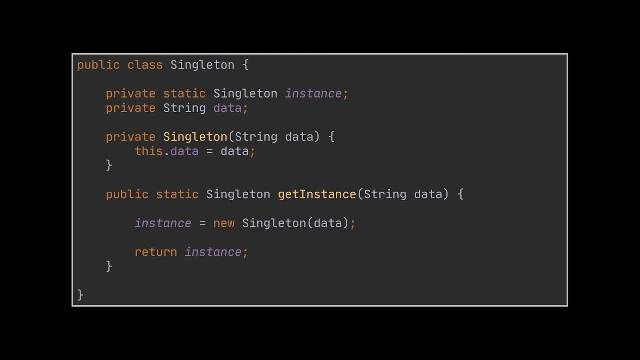 at the beginning of our implementation. But how do we guarantee that the same instance isłam Instance is вполне double completion. But how do we guarantee that the same instance is simplesmenteliamo application, now that the method allows for returning a statement of a Singleton? 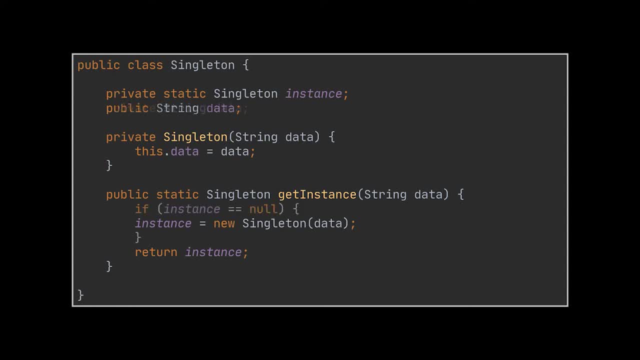 is returned every single time. Well, the created instance is wrapped inside an if statement that checks if the static instance of our singleton is null or not, and only if it is, we proceed by creating a new instance of it using our private constructor. However, if it isn't, we return the. 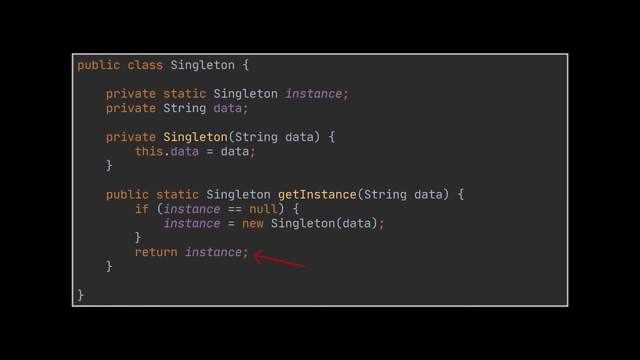 same instance already stored inside our singleton class. Now some of you may say that the code we wrote isn't robust enough, because if we were dealing with multi-threaded environments, nothing in this code prevents two threads from accessing this piece of code at the same time and return. 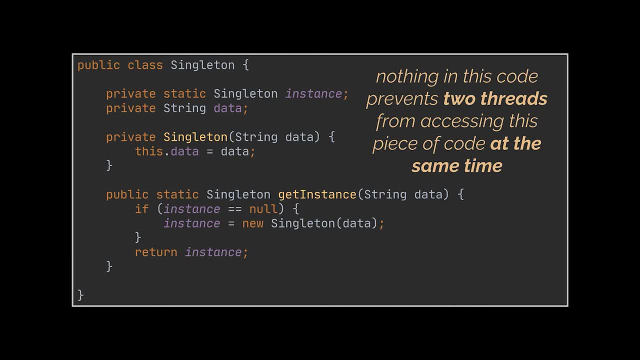 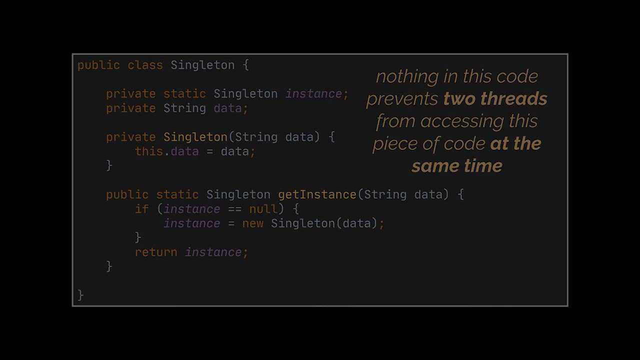 with two different instances of this same singleton class, And to these people I say: you're right To solve this issue and, as discussed in our previous videos, all we have to do is wrap our if statement with a synchronized block. Now, every time a thread tries to create an instance of the 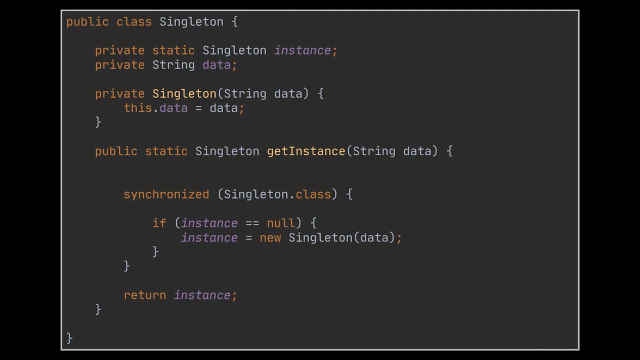 singleton class. it will have to wait for its turn, as one thread only may execute this code block at a given time. Okay, with this we solved the threading issue. However, we added unnecessary overhead to the creation process of our singleton object. You see, after this single instance is created, when the threads 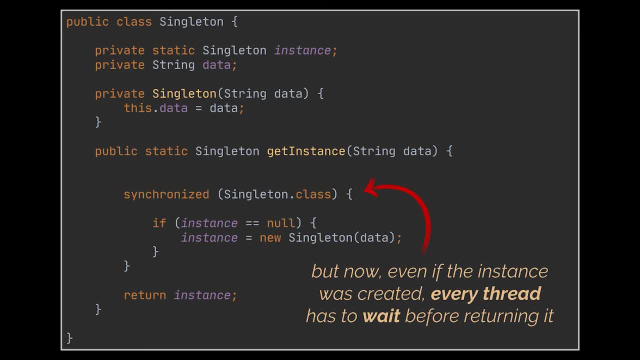 of our application try to access it, they will first have to wait for their turn to acquire the lock on our class and only when it is their time to go they will check if the instance is available and then return with it. This problem is actually not specific to the singleton pattern and can be. 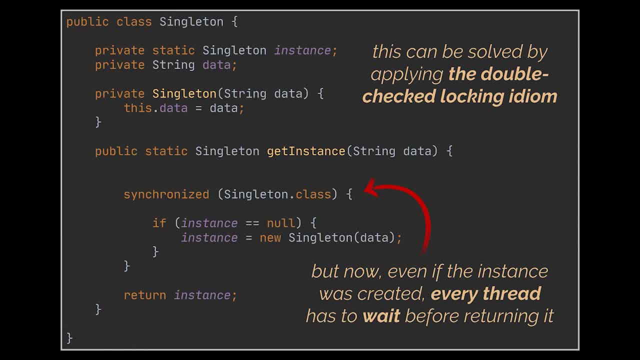 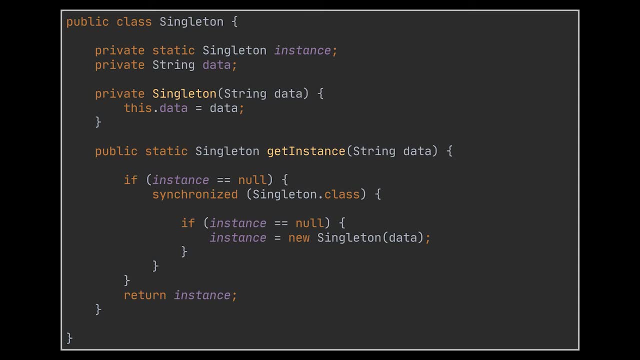 solved by applying the double-checked locking iGEM on our method. How do we do that? Well, we simply wrap the synchronized block with another if statement similar to the one inside it. I know the code may look confusing at first, but look. 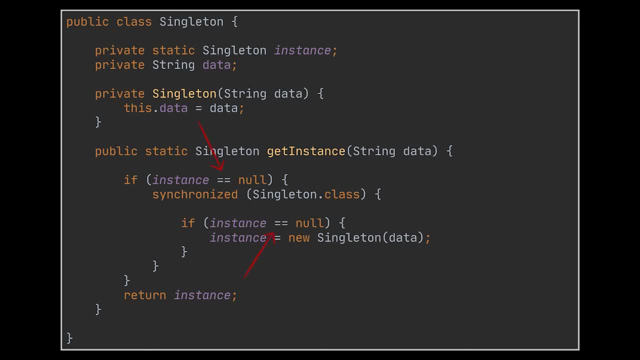 closely. Now. the threads trying to retrieve the instance of our singleton class after being instantiated do not necessarily have to acquire the lock on our class, as we are first testing the locking criterion. What we did improved the performance of our code by limiting synchronization. 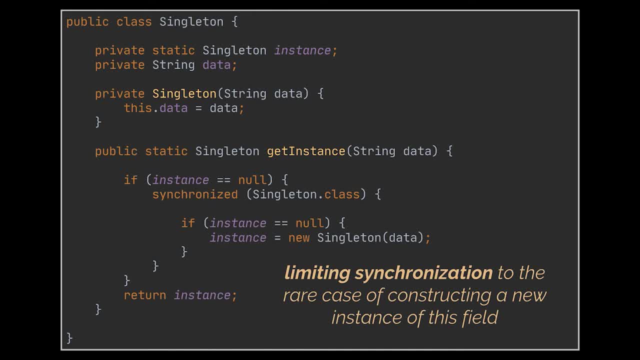 to the rare case of computing the field's value or constructing a new instance of this field, and by skipping synchronization during the common cases of retrieving an already created instance or value of this field. Okay, intuitively, this piece of code may seem like a complete and efficient. 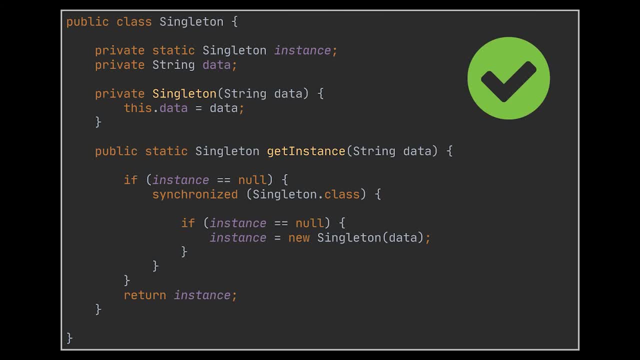 solution to the multi-threading problem we were mentioning. However, it is still missing something. Consider: we have two threads in our application trying to access this method, threads A and B. Thread A is the first to access the method and it notices that the instance of our singleton is not. 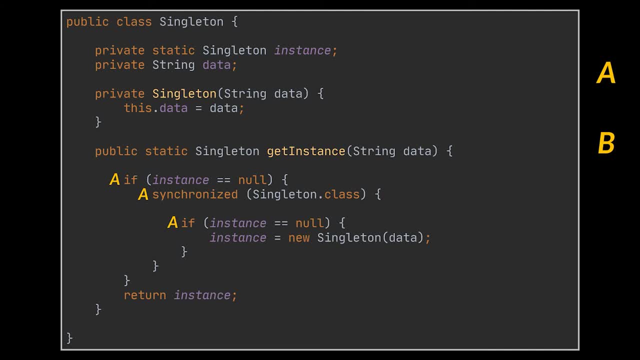 initialized. Therefore it obtains the lock and begins to initialize the value. Now, due to the semantics of some programming languages, the code generated by the compiler is allowed to update the shared variable stored in the memory to reference a partially constructed object. So, 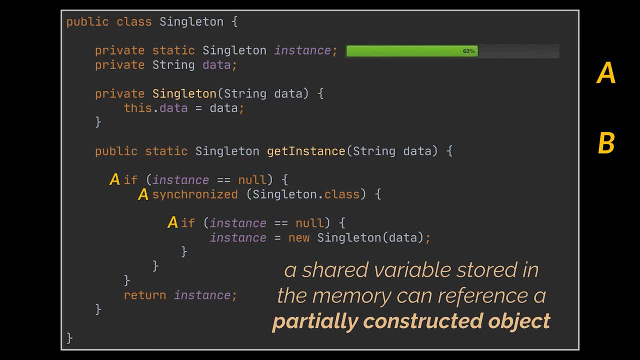 before thread A finishes the whole initialization process. the shared variable, or the singleton in our case, can be Sarah today and we will need toantically send significant value from the single term into the Internet to our trying case. As a psychologist I have decides what our 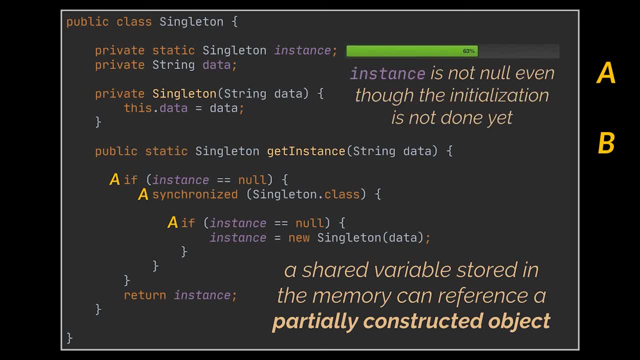 standard of novel emocional data is such as using a feasiblecka brane assisting another thing to convince updated in the memory, and other threads of our application will consider it as initialized and use it. In our example, while this object is being constructed by thread A, thread B may try to. 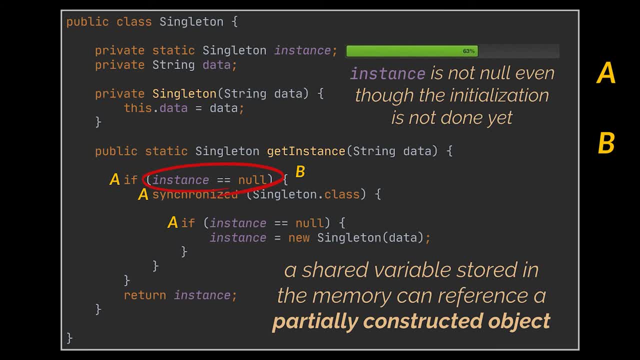 retrieve it and, because of the first if statement we just added, thread B will not wait for thread A to finish the initialization and will use the instance referenced, even if it is a partially constructed object, causing our application to crash. To avoid such scenarios, all we have to do 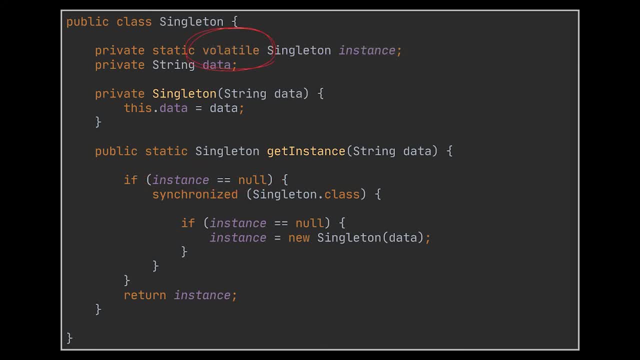 is set the singleton instance, we have to be volatile. This keyword ensures that multiple threads will be able to handle the singleton instance correctly. If you have no idea what volatile fields are, or if you haven't made use of this keyword before, feel free to check the video. 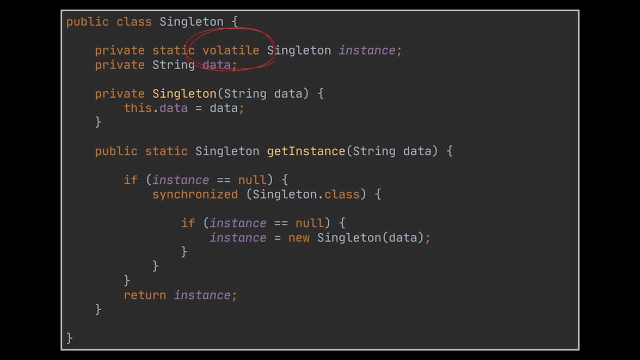 linked down below in the description. Now this is a complete and working solution for the singleton pattern. Additionally, there is some kind of a micro-optimization we can do to enhance the performance of this implementation. You see, the variable we have is now marked as volatile. so every time we access this variable, we need to 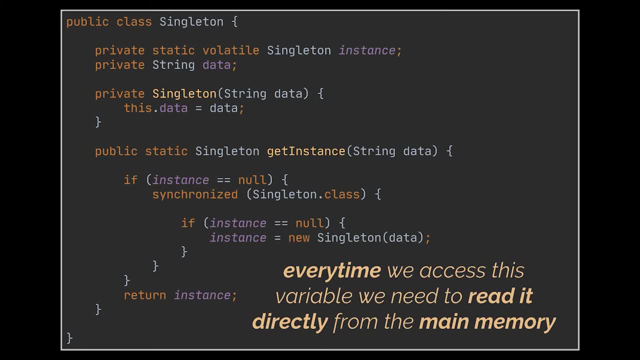 read it directly from the main memory, as it cannot be cached. So in this single code snippet, even if the variable was already initialized, we have to fetch it twice, The first time in the if statement to check if it is null, and the second time in the return statement to return it to the user. 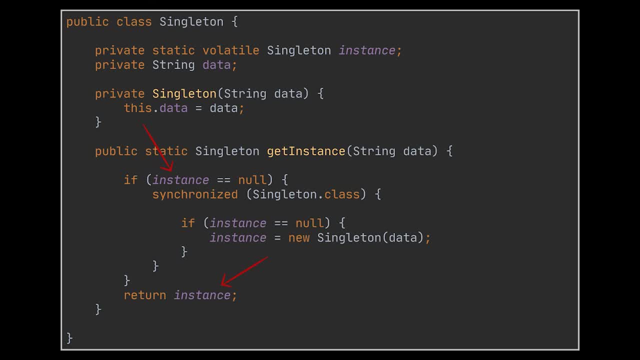 To avoid doing this and access the memory only once. what we can do is store this instance in a local variable the first time we return it to the user. To avoid doing this and access the memory only once. what we can do is store this instance in a local variable To avoid doing this and access the memory. 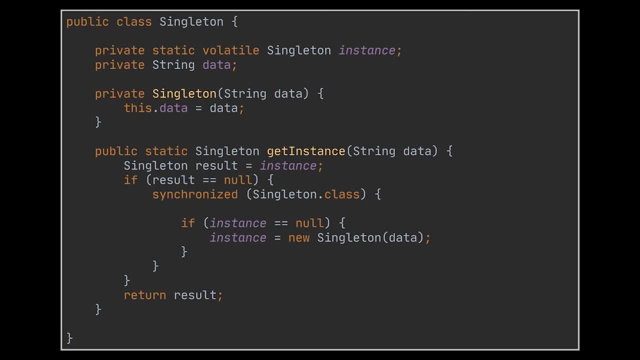 only once. what we can do is store this instance in a local variable the first time we return it to the user. Then use this same local variable in both the if statement and the return statement. The same logic and way of thinking can be expanded and used inside the 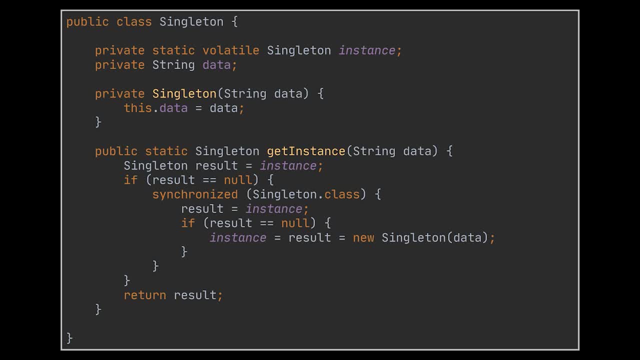 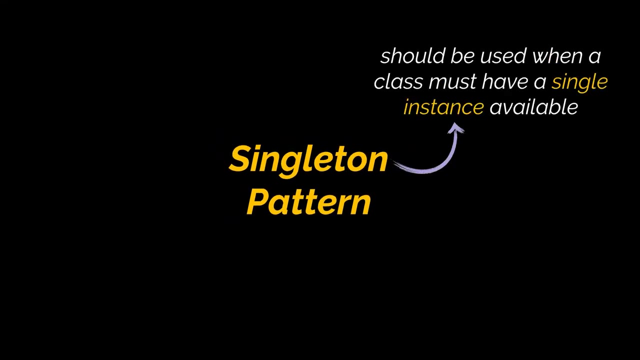 synchronized blocks to avoid multiple direct reads of the memory. This simple usage of such a local variable can and will improve the method's overall performance by as much as 40%. so to recap, we can say that the singleton pattern should be used when a class must have a single. 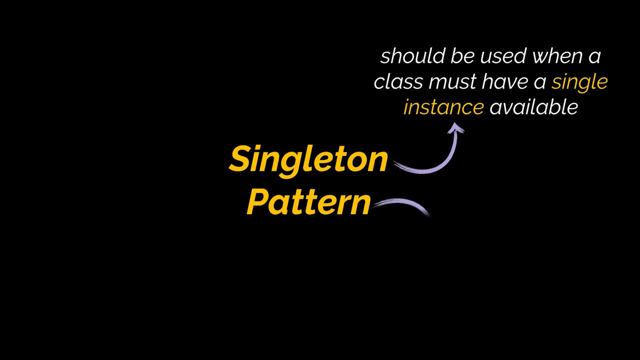 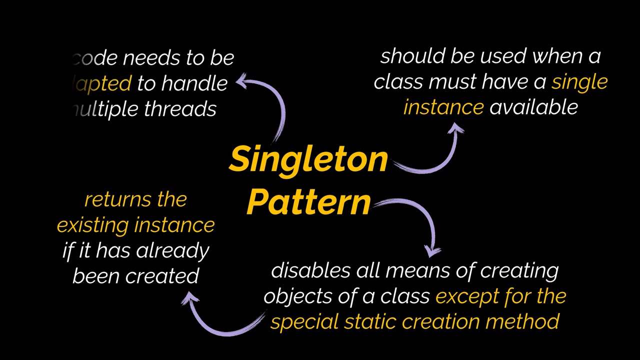 instance, available to all its clients, as this pattern disables all other means of creating objects of a class, except for the special static creation method. This method either creates a new object or returns the existing one if it has already been created. However, this pattern requires special treatment in a 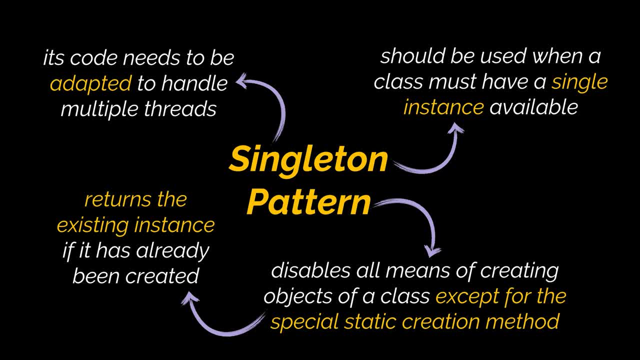 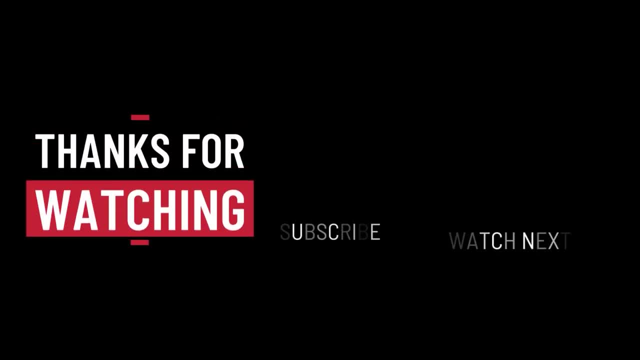 multi-threaded environment, as its code needs to be adapted to handle multiple threads. So that's it for this video. I hope it was helpful. Thank you guys for watching. take care and I will see you in the next one.